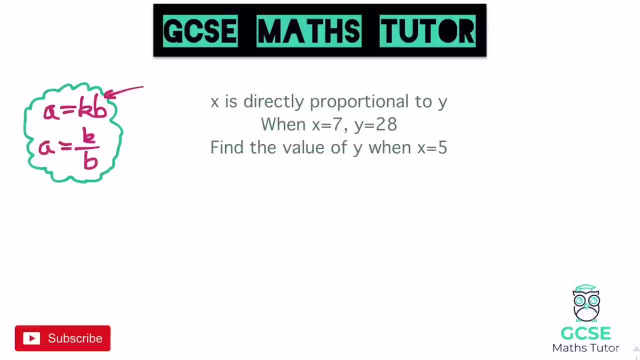 a equals kb. We're going to write that pretty much for all of these. Okay, so we've got a x and y in this. We're going to have x equals k, lots of, or k times y. Okay, we're just going to find out what y is actually being multiplied by to make x. So it says in the next line: 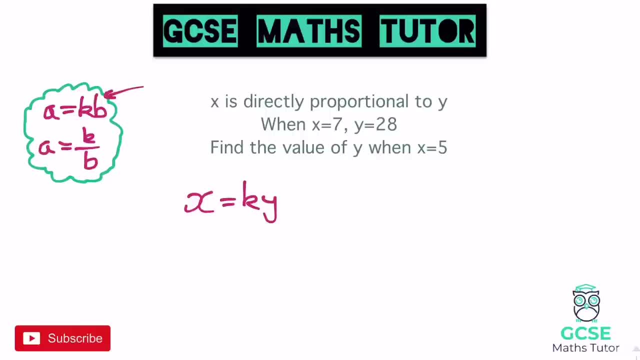 when x is 7, y is 28.. So it gives us two of the values here and if we plug those values in, we're only going to have one unknown, being the k, which means we can definitely solve it. and we can solve any equation when there's one unknown, unless of course, we're looking 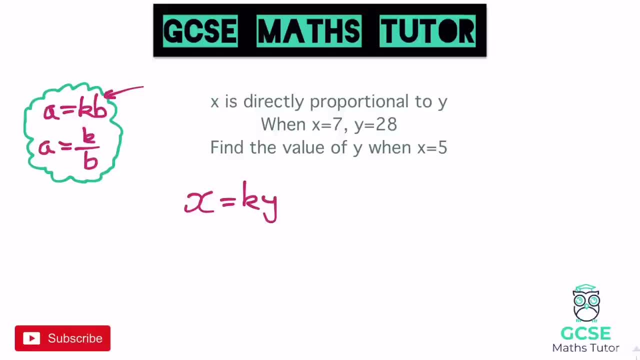 at simultaneous equations and beyond, in which case we might have two unknowns, But in this case we are going to just ensure that we only have one unknown in our equation. So we're going to find the value of y when x is 5, and I'm going to ignore that for the moment, because 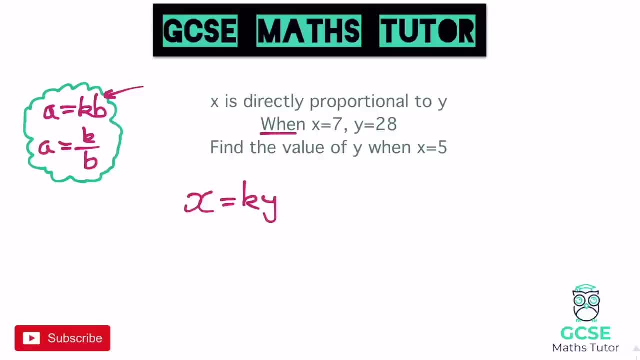 I'm going to find out what k is first based on this first bit of information here. So when x is 7, y is 28.. So if I plug those in, x is 7 and that's going to equal k lots of, or k times 28.. Okay, now I'm going to rewrite this in a slightly different way, Rather than 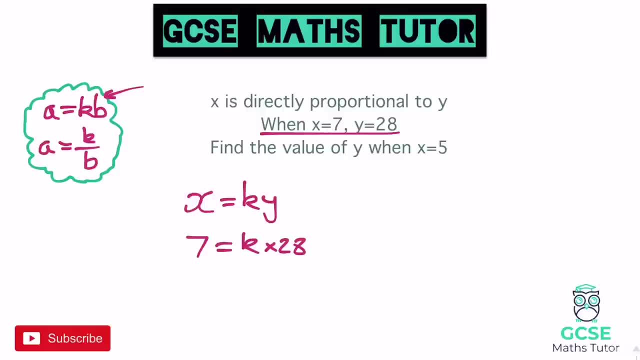 writing k times 28. I'm going to write 28k. Okay, I'm not going to write out that step like that in any of the other questions. I'm just going to write it as 7 equals 28k, because we're used to seeing it like that. We quite like it looking like that. Okay, so for the 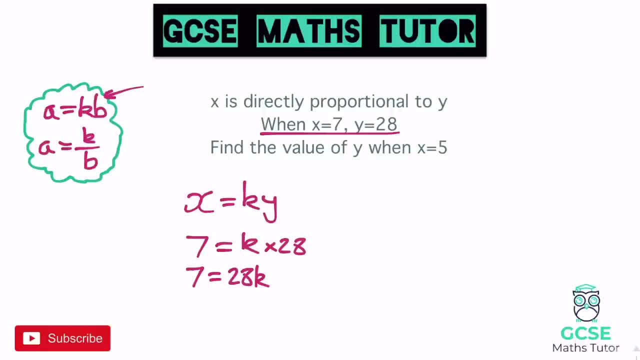 next one for the next step. here we need to actually solve this. So if it's 28, lots of k, we need to divide both sides by 28.. So we've already got one. that's not very nice in our first question here. So 7 divided by 28 equals k, Obviously, if you've got a calculator, this 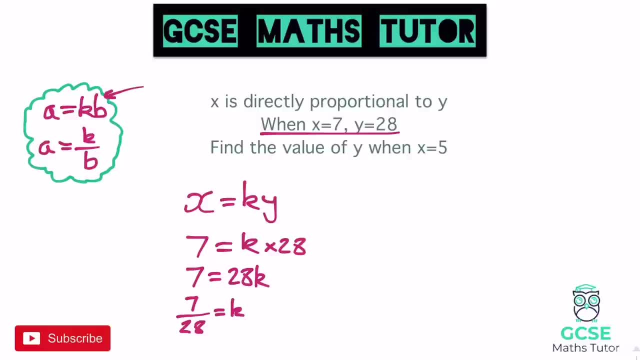 is quite nice. Okay, if not, you are just going to have to simplify that as a fraction: Top and bottom both divide by 7.. So actually, if we just simplify it without a calculator, 7 on the top is 1 and 28 divided by 7 is 4.. So it's one quarter or 0.25.. And you can write: 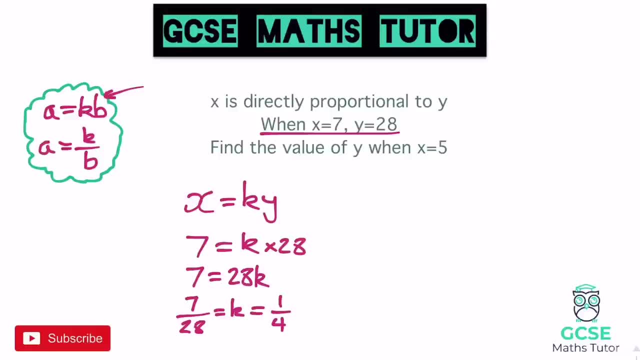 it as a fraction or a decimal, obviously. if you've got a calculator here, This is obviously quite nice. So if we rewrite our formula- and this is what we always have to do- We've found k now, so we can actually replace k in this formula that we're going to be using throughout. 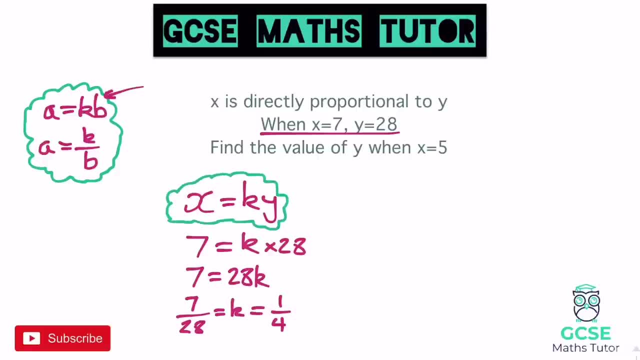 the question, And we can just write that k as being one quarter. So let's go for that. x equals one quarter y, Or in other words y is being multiplied by a quarter To find the value of x, And you can probably see that on this one, as we've not got any. 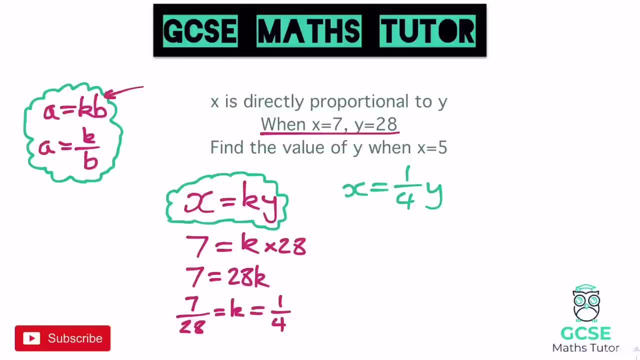 further little bits going on here happening to the y. It's actually quite nice to see that there. So y is being multiplied by a quarter to get x. So if we plug this next value in, it says: find the value of y when x equals 5.. Now what we have here is a formula. 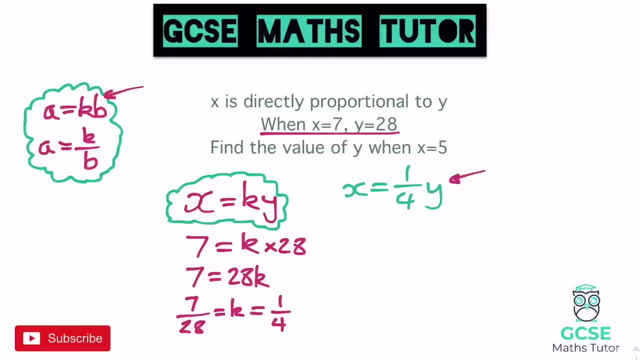 to work out x in terms of y, And all that language means is we've got x equals something, y. Okay, so it's a formula for x in terms of y, And you might just be asked to write down a formula. So it's just x in terms of- and I'm not going to write this down on every question, but there 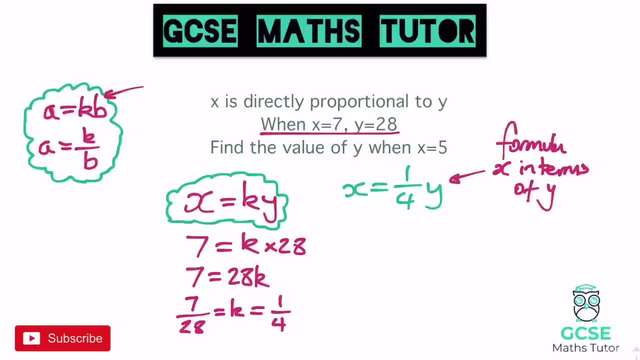 we go. that is a formula for x in terms of y. Okay, so all we've got now is we've got find the value of y when x is 5.. So if we plug 5 in, we get 5 equals a quarter multiplied by y. Okay, so basically, what number can you quarter to get the answer 5.. Now, hopefully, 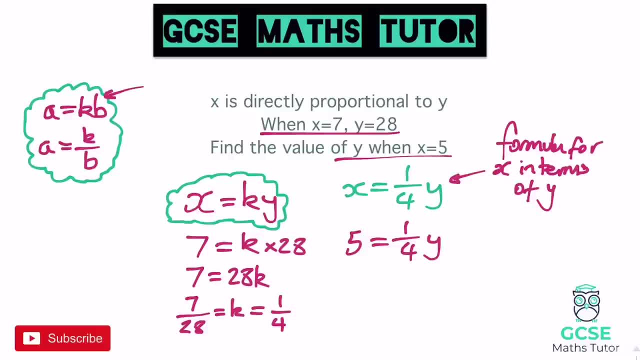 you know the answer: there is 20.. It's a quarter of 20.. 20 is 5.. But if we just follow our normal solving equations approach here, we divide both sides by a quarter, There you go. Divide by a quarter, There you go, And obviously 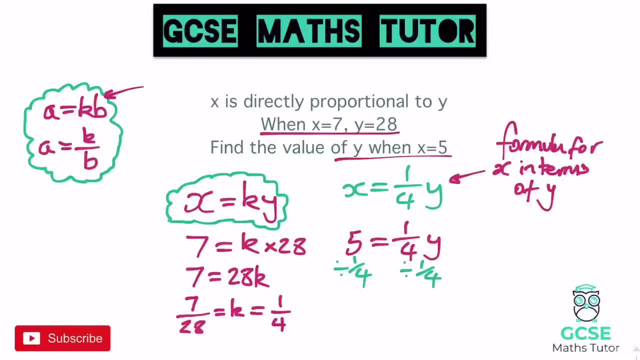 if you've got a calculator again, you can just type in 5 divided by 0.25 or you can just think logically here: a quarter fits into 1 four times, So it fits into 5, four lots of that, or 20 times. So when you divide by a quarter you get 20 equals y, Or obviously. 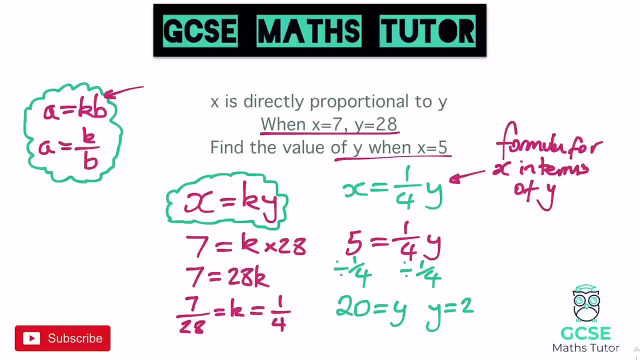 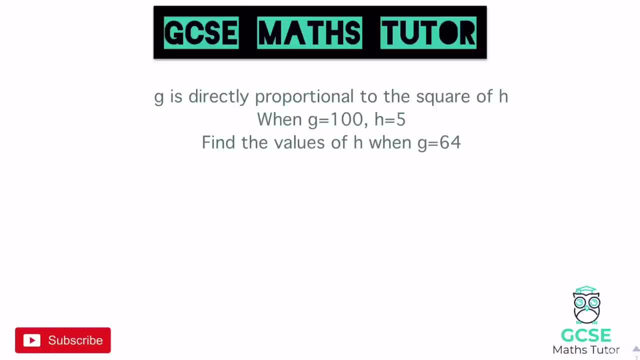 you could write that y equals 20.. And there is your first answer for this question here. Let's have a look at another one. Okay, so for this question it says G is directly proportional to the square of H. When G equals 100, H equals 5.. Find the values of H when G equals 64. Now we'll address this values. 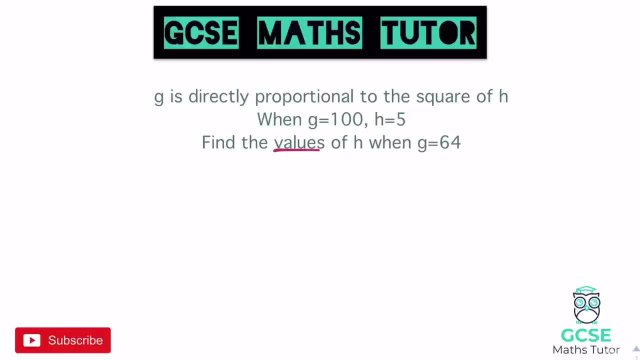 aspect here in a sec as we move on. But let's just go with our normal formula here. So G equals KH. Now I've got to make a slight amendment here, because it doesn't say G is directly proportional to H, It says the square of h. 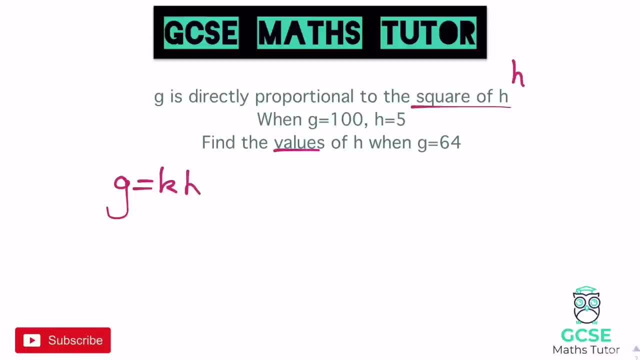 So the square of h just means h squared, which could be written like this: It could just say directly proportional to h squared. So in our formula we just need to add our little squared there with the h And we're going to treat it in exactly the same way and just sub these numbers in. 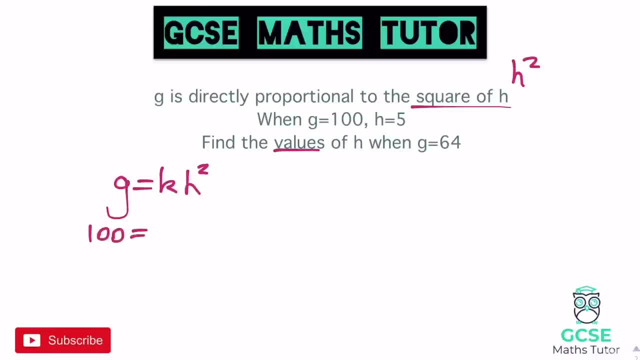 So it says: when g is 100,, so g is 100, and that equals- and let's work this out to the side: Look, h squared. well, 5 squared is 25.. There you go, So I'm just going to work that out straight away. 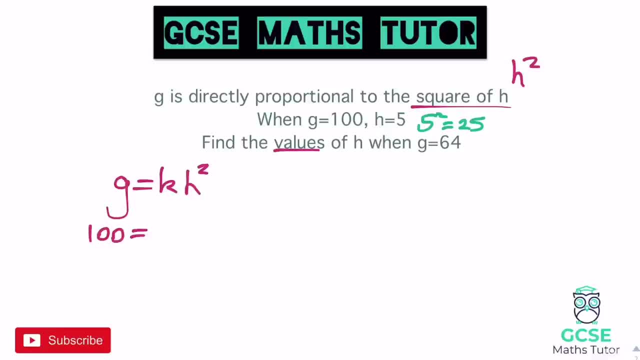 That's the number I'm going to put in instead, because it's h squared. So rather than putting k times 25,, I'm just going to put 25k And then solving this just like we would in a normal equation: divide by 25, and we get 4 equals k or k equals 4.. 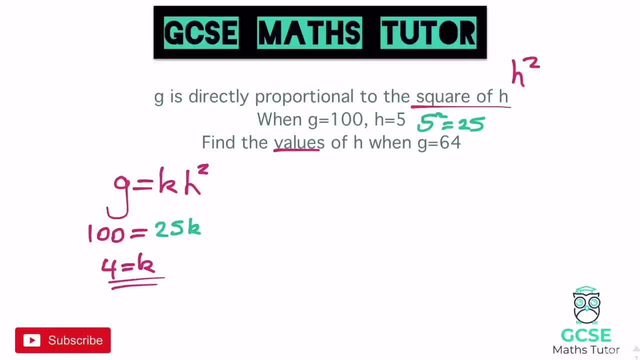 Now put that back into our little formula. So we've got k is 4 now, so we can put g equals 4h squared rather than kh squared, And then we just need to sub in our new value. So find the values of h when g equals 64.. 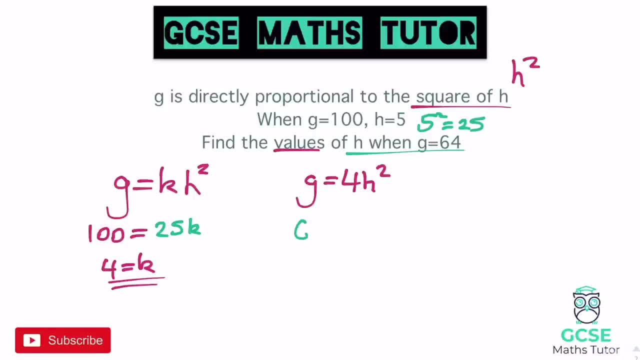 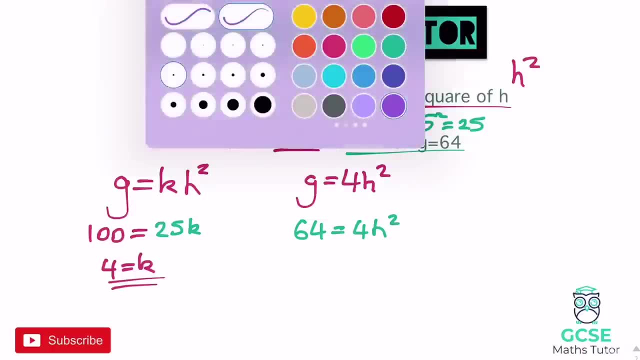 And if we sub that in, let's have a look: 64 for g Equals 4h squared. And again, we just need to solve this Now. we can't square root yet. We need to get rid of this 4 first. that's stuck onto the h squared. 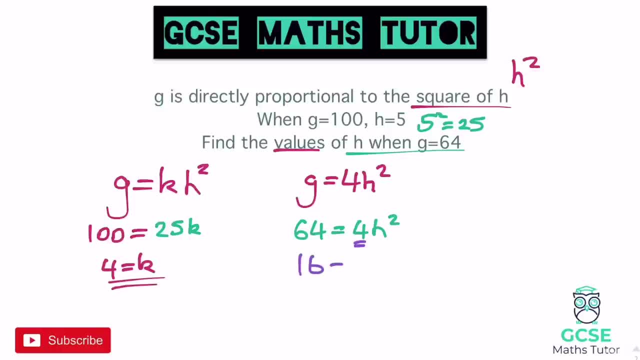 So if we divide both sides by 4, we get 16.. So 16 equals h squared, And to find the value of h we're going to have to square root both sides, because that's h squared and the reverse of squaring is square rooting. 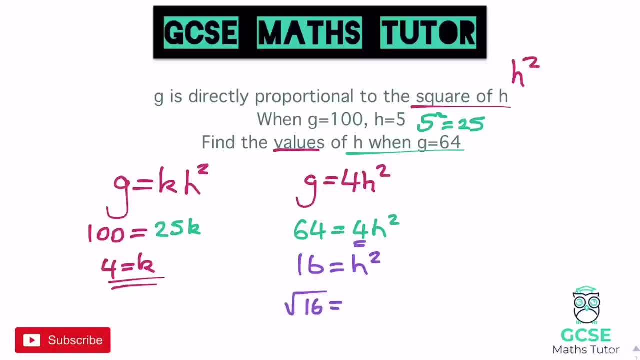 So we're going to do the square root of 16, which is going to equal h. Now, this is where this word values comes in. Again, this is something that is quite important, Because there is two square root answers to 16.. 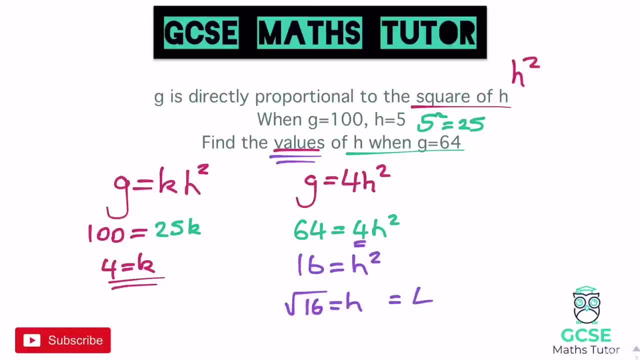 Obviously, hopefully you know, the square root of 16 equals 4.. But it also equals negative 4.. So I would have two answers here. It could be positive 4 or negative 4.. That's why it says: values 4 times 4 is 16, and negative 4 times negative 4 is also 16.. 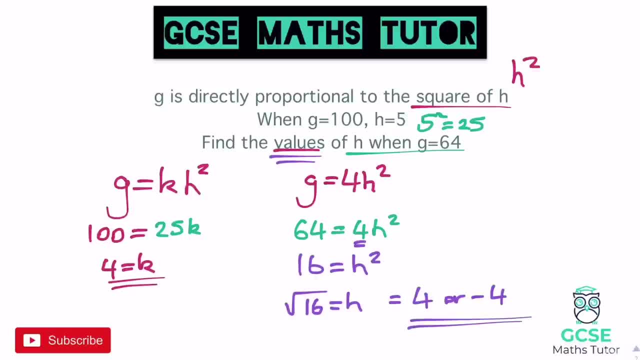 So whenever your square root's a number, you've always got the positive and negative version there. So we get two answers for this question. Let's have a look at one more before we have a go. Okay, so the last question here. 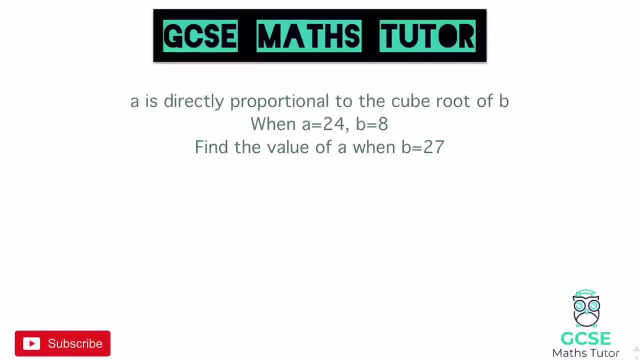 Okay, Cube root of b, So cube root of b, and that can also be written like this: Cube root of b. So let's write this in: a equals k, cube root b, And let's plug in the value, So a is 24.. 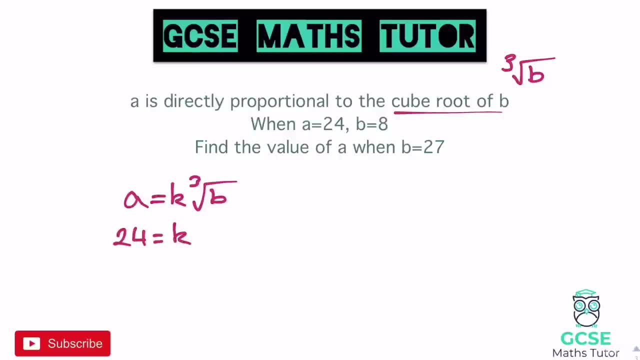 So 24 equals k cube root of b, And I'm going to work this out to the side because that's the cube root of 8.. And the cube root of 8 is 2.. So I'm going to put 2k in there. 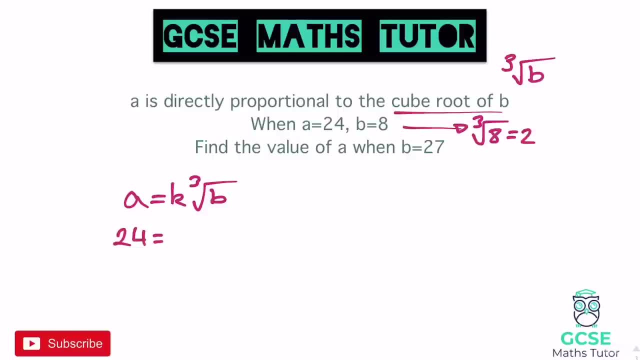 I've already put my k in, so we might have had to rewrite that. Let's have a look. Let's get rid of that. 2k. Divide both sides by 2. And we get k equals 12.. There we go. 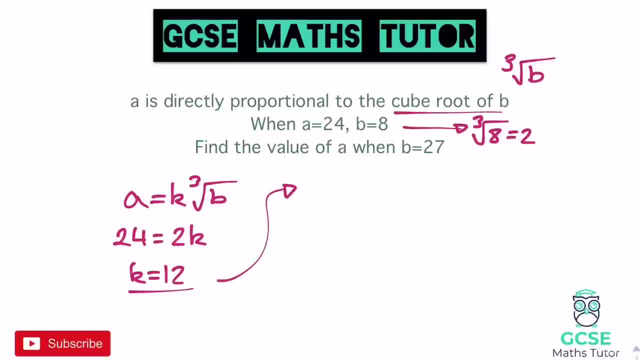 We've got our value of k. Let's rewrite our formula. Let's bring that back up And we get: a equals 12 lots of the cube root of b. Now again onto that last line. It says: find the value of a when b equals 27.. 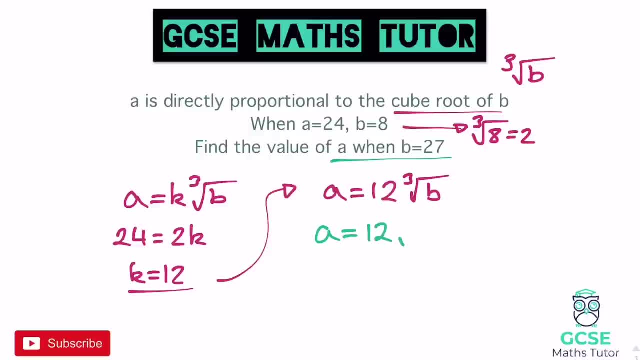 So let's plug that in a equals 12 times the cube root of 27.. There we go. The cube root of 27 is 3.. So it's 12 times 3. And that gives us a final answer there of 36.. 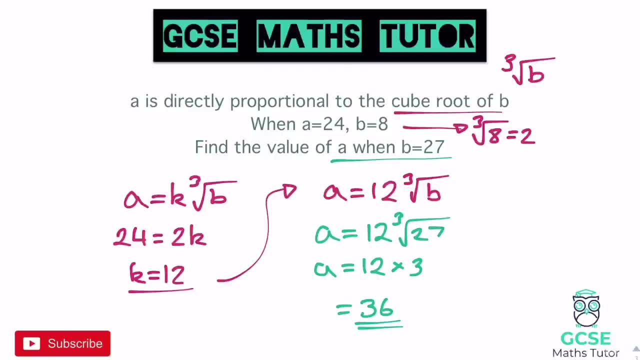 So we've got a very, very similar process in all these questions. It gives us two values, We sub them into our little formula. Always looks very, very similar. We just use this idea- a equals kb- And obviously just amend the b there. 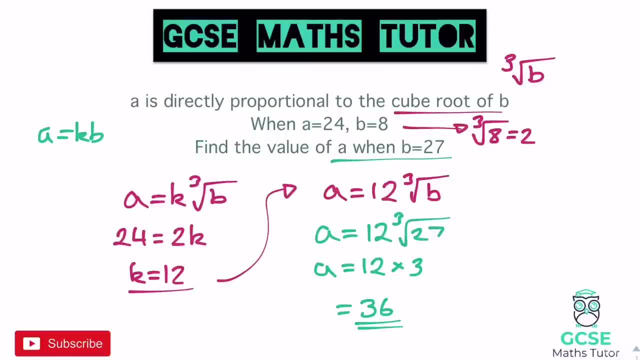 If it's a b- squared, or a root b or a cube root or a cubed, you just stick that with the b and just treat it as normal, Obviously amending the number there when you sub it in. Once you get the value of k, put it back into your original formula here. 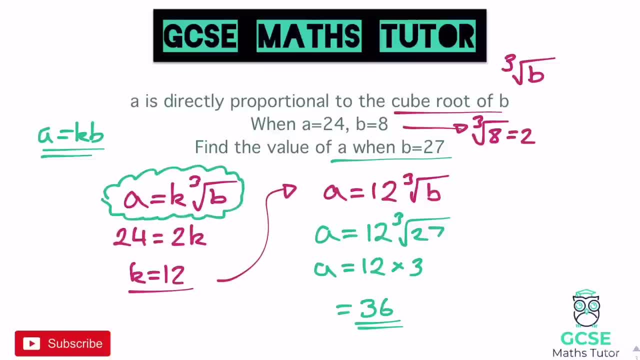 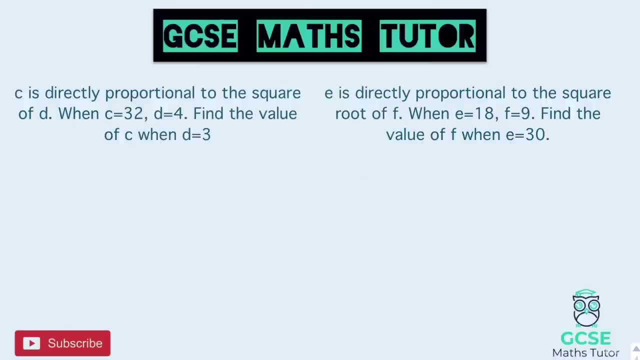 Okay, You're going to use this throughout the question And then just re-solve your equation using the new value to find that other unknown. Okay, So here's some for you to have a go at. Okay, So two questions there. 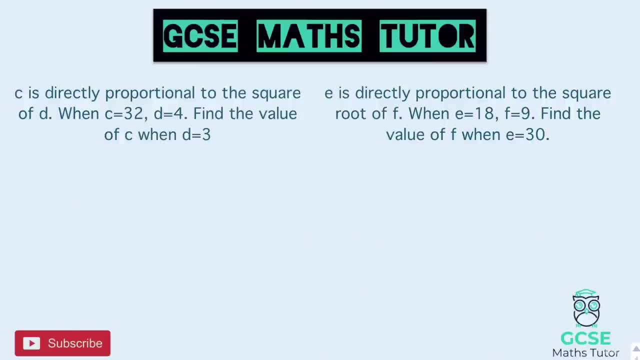 Pause the video. Have a go. I'm going to go over the answers in a sec. Okay, So c is directly proportional to the square of d, So c equals k. That's a bit of a rubbishy k. There we go. 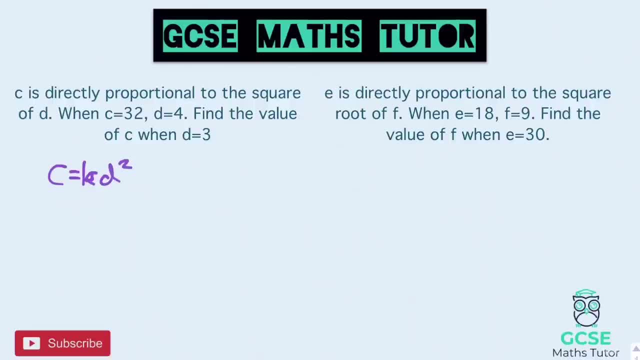 k d squared. Okay, The square of d When c equals 32.. So 32 equals kd squared. So 4 squared is 16.. So 16k. There we go, 16k And divide both sides by 16.. 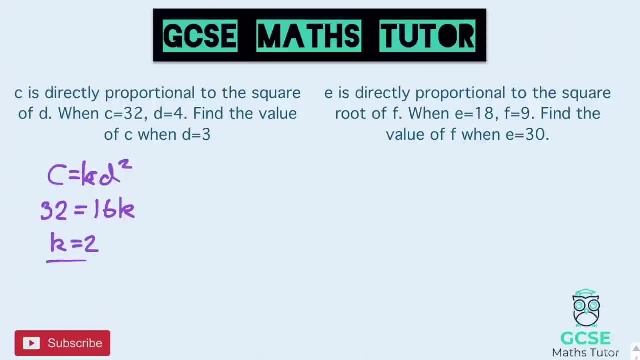 You get: k equals 2.. Right, Let's sub that back in. So c equals 2d squared. And then find the value of c when d equals 3.. So c equals 2 lots of 3 squared, which is 9.. 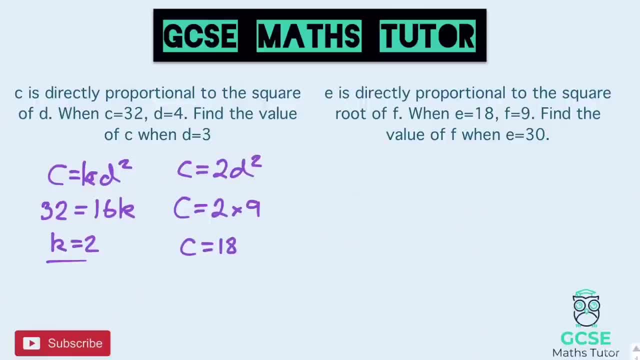 So 2 times 9.. So c equals 18. there And there's our final answer. On to the second question, Let's have a look at this one. e is directly proportional to, So e equals k Square root of f. 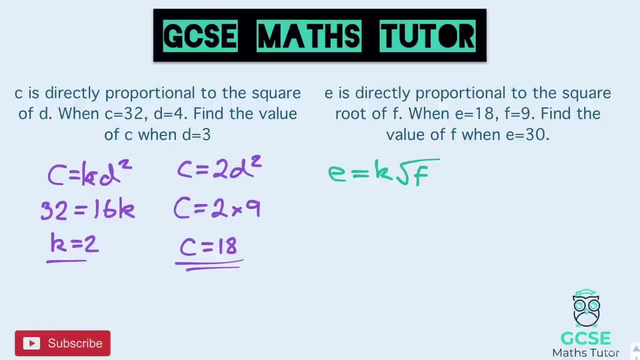 So root f When e equals 18.. f equals 9.. Find the value of f when e equals 30. So when e equals 18. We have 18.. Equals k root f. The square root of 9 is 3.. 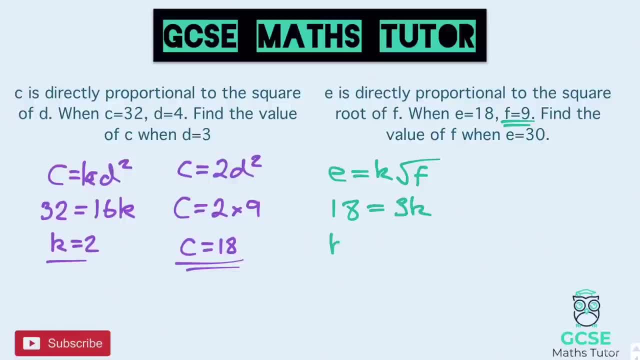 So 3k, Divide both sides by 3. And we get k equals 6.. Sub k equals 6. back into our formula. So e equals 6 root f. And then what have we got? We've got Find the value of f when e equals 30.. 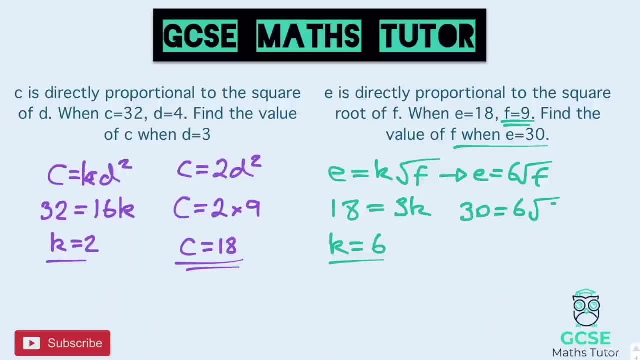 So 30 equals 6 root f. There we go. Divide both sides by 6. We get 5 equals the square root of f. And then we need to square both sides, this time to get rid of the square root. So square both sides. 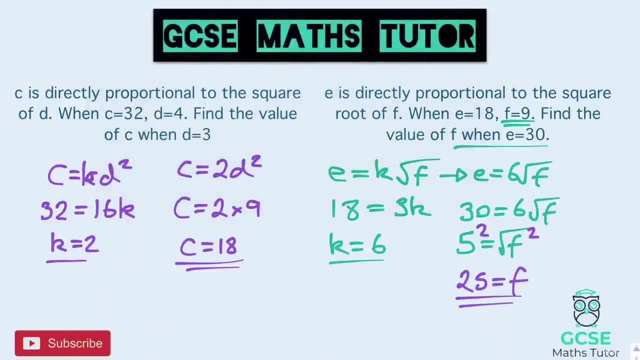 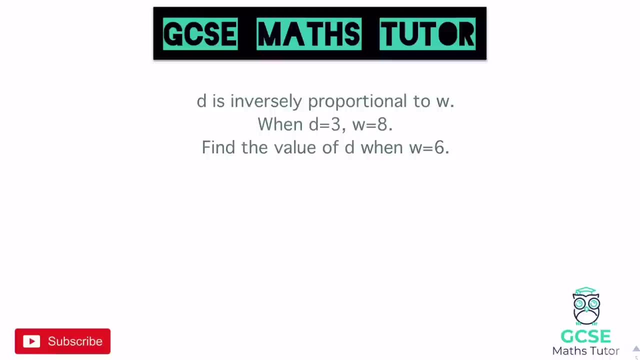 And we get 25 equals f or f equals 25 is our final answer. Right, there we go. There's direct proportion. Let's have a look at some inverse proportion. Okay, so we talked about the formula for this at the start. 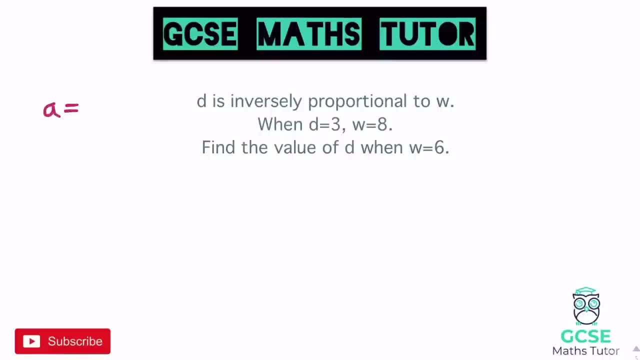 So rather than using A equals kb, This time for inverse proportion We use a equals k over b. So looking at our values here, It says D is inversely proportional to W. So I'll plug the values in: D is inversely proportional to W. 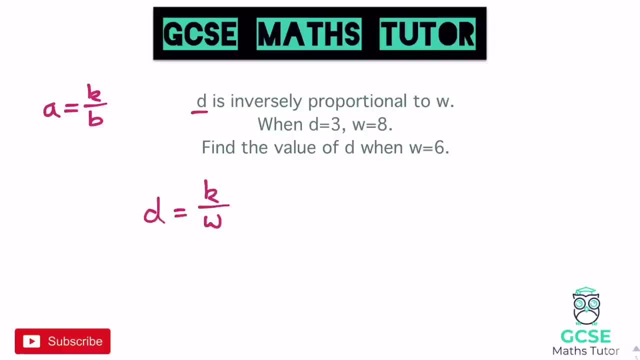 So k over W, And you always put that first letter as the equals. So D equals, and then whatever it's inversely proportional to, Which just means our constant is being divided by W in this sense. Okay, so it's just two formulas that you need to know here. 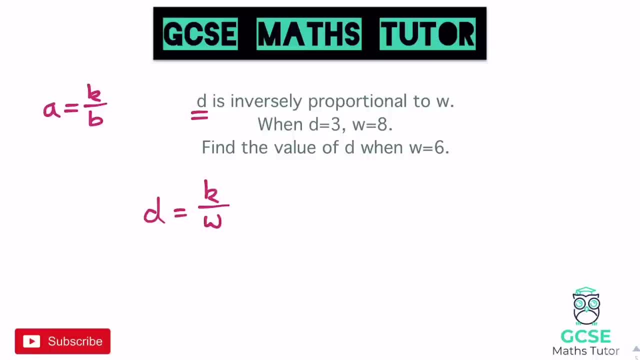 So this is when D equals 3.. W equals 8. We treat it in exactly the same way. So 3 equals k over 8.. And then again solving that to find k. So k is being divided by 8.. So times both sides by 8 and you get 24 equals k or k equals 24.. 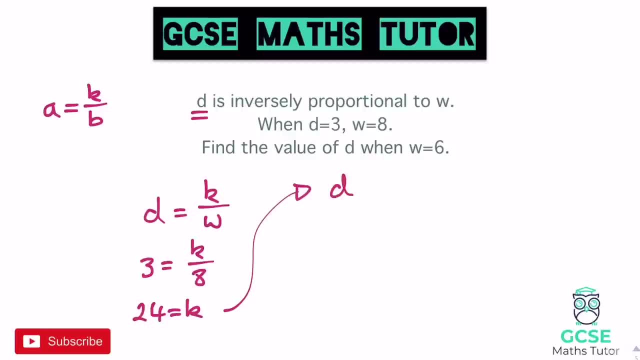 Again. bring that up to the top, Plug it back into our formula and we get: D equals 24 over W, And then we just need to sub in our final value here, So find D when W equals 6.. So D equals 24 over 6 and 24 divided by 6.. 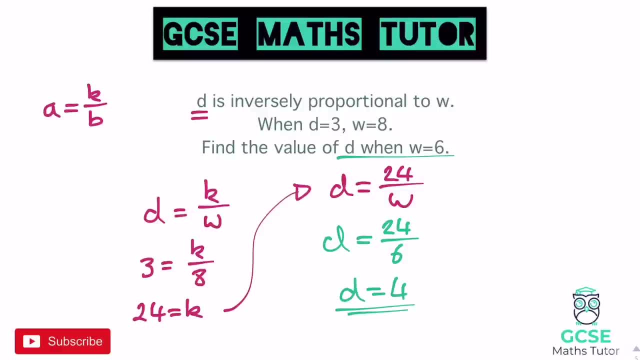 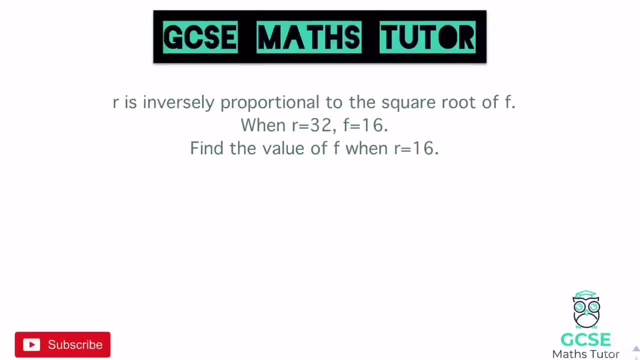 Leaves us with 4.. So D equals 4 as our final answer. Okay, so there's some inverse proportion. We're going to have a look at another one. So R is inversely proportional to the square root of F. So square root of F obviously a little bit different here. 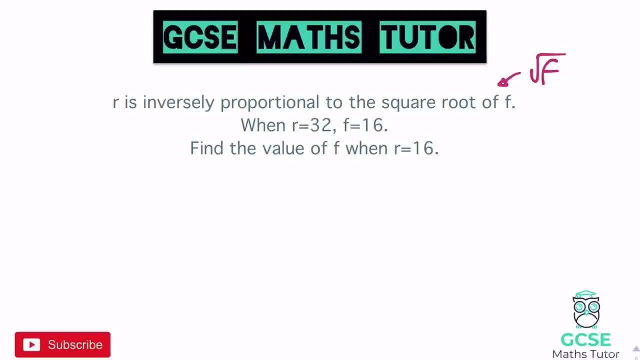 You've got to take note of this. Root F When R is 32,, F is 16.. Find the value of F when R equals 16.. Okay, so don't just assume that it's going to change in a certain way here. 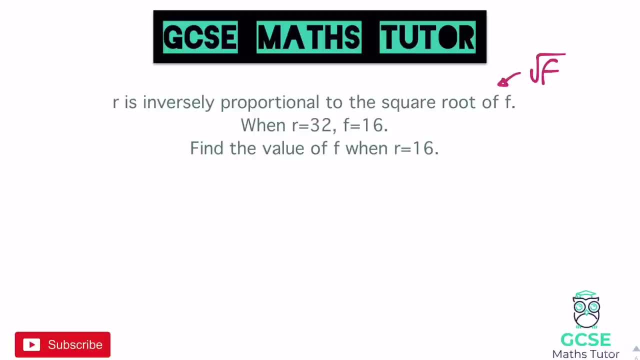 Because 16 is half of 32.. R is being halved there. Let's actually just have a look and see what happens. So R equals k over 8. K over the square root of F, And let's plug in these first two values. 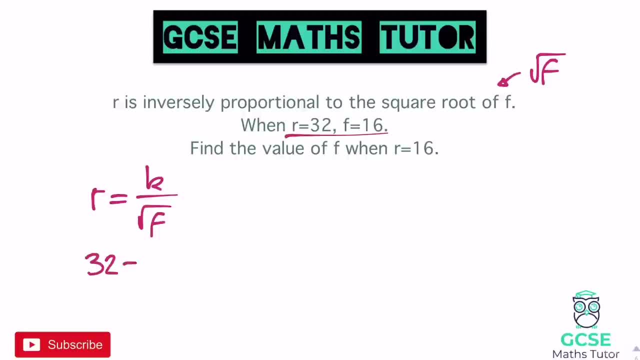 So 32 and 16.. So 32 for R equals k over the square root of 16.. The square root of 16 equals 4.. So we can work that out and save ourselves writing it down lots of times. So k over 4.. 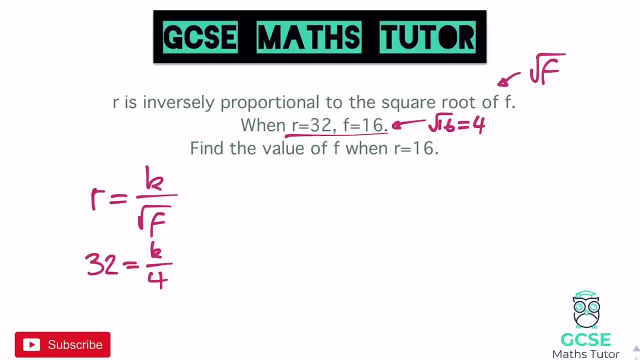 Multiply both sides by 4 here to remove that divide by 4.. And 32 times 4 is 64.. 128.. So 128 equals k, Again exactly the same as before. Let's plug that back into that original formula. 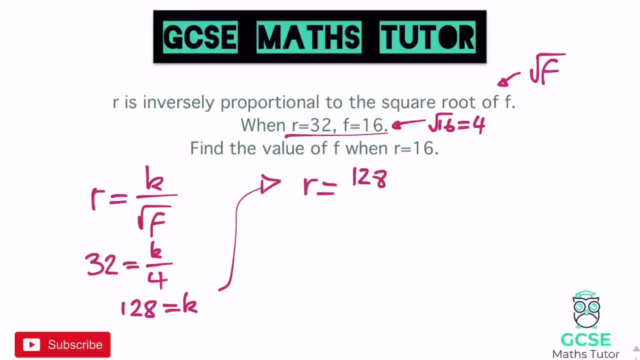 So R equals 128. now over the square root of F, And then, finishing it off, let's plug these last two values in, Or the last one value. So find the value of F when R equals 16.. So let's have a look. 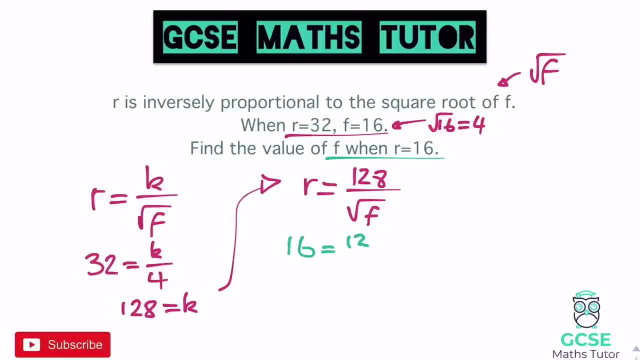 We get 16 equals 128 over the square root of F. Now this is definitely one of the hardest scenarios here, Because we've got to rearrange this now. So there's a And there is a nice little quick trick. We can just swap the 16 and the root F. 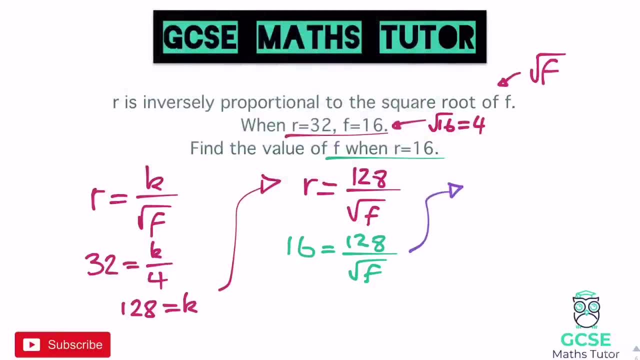 But if I just do this in two slow steps. So first things first, If we multiply both sides by root F, we get 16. lots of root F, Or 16 times root F equals 128. And then you can divide by 16.. 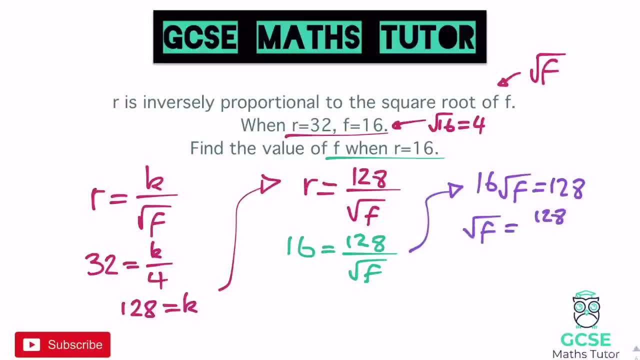 And you get the square root of F equals 128 divided by 16.. Okay, so it's two steps there, And you can quite happily just take those two steps, But you can actually just swap these round, Okay, if you just think about the logic there in terms of what you're doing. 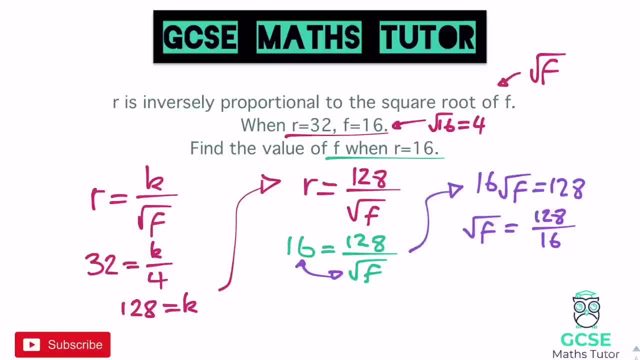 Times it over and then divide the other one. You can just swap them over. So we get the square root of F equals 128 over 16. And you might be looking at that thinking that it doesn't divide. Actually, 128 does go into 16.. 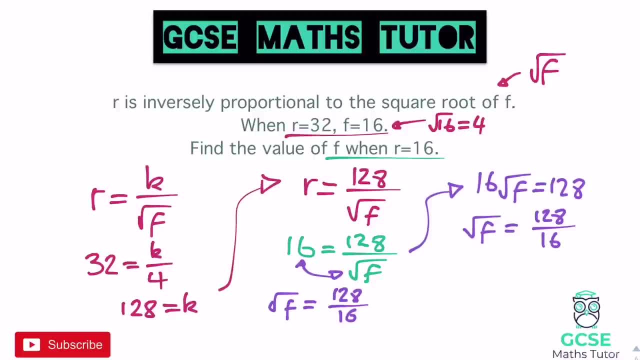 If you didn't have a calculator, You just have to build that up and work your way up to 128.. Writing down the 16 times table. Obviously, if you do have a calculator here, this is quite nice. So that ends up being the square root of F equals 8.. 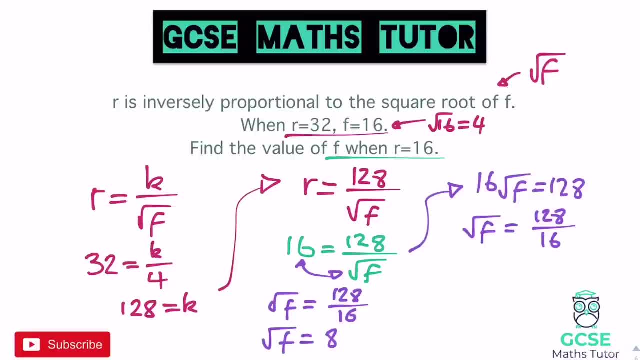 128 divided by 16 is 8.. And obviously here that is the square root of F. To square both sides to finish this off, To find out what F is. And 8 squared gives us F equals 64.. Okay, so very, very similar process, obviously. 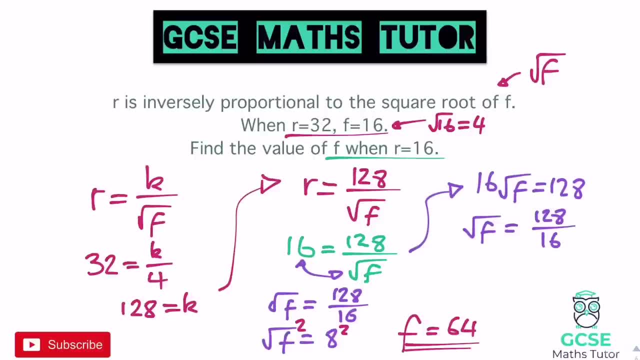 But we're looking at inverse proportion. So you've got K over whatever this second element says, it is here The square root of F, or F squared or cube root of. Okay, you just stick that in and just treat it like an normal number there. 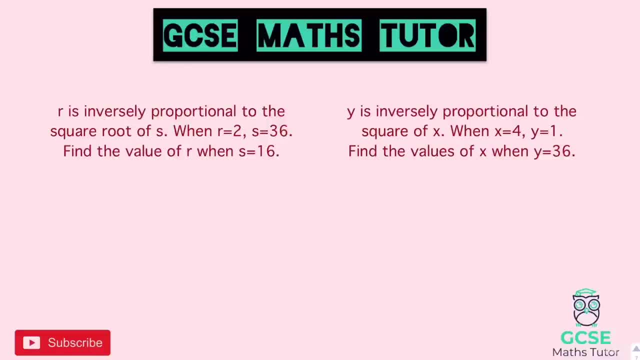 So here's something for you to have a go at. So here's two questions. Pause the video there. We'll go over the answers in a sec. Okay, let's have a look then. So R is inversely proportional to the square root of S. 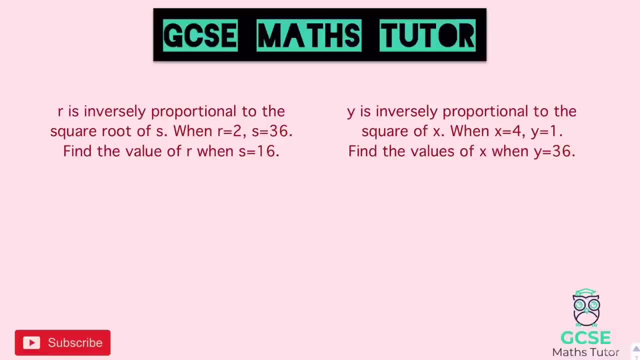 When R is 2, S is 36.. Find the value of R when S is 16.. Okay, let's start writing this down then. So R equals K over the square root of F. So root S. It says: when R is 2, S is 36.. 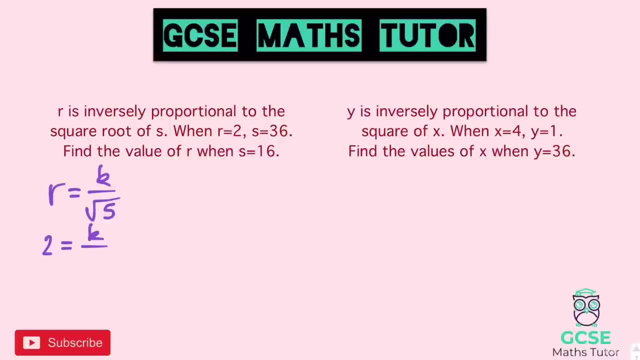 So 2 equals K over and the square root of 36. Let's just write it here- is 6.. So K over 6 times both sides by 6. You get 12 equals K or K equals 12.. And we can plug that back into our formula here: 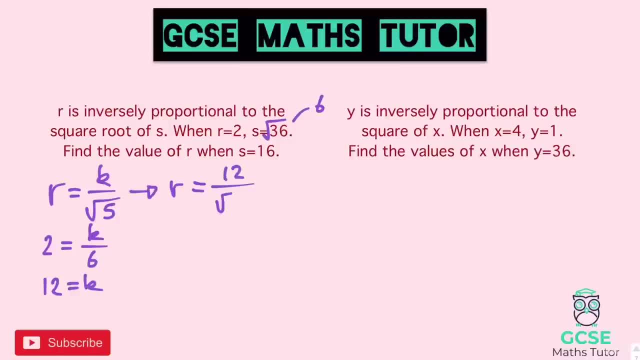 So we get R equals 12 over the square root of S. I never like writing these S's down. They always look like fives, So just make sure you don't get confused about what you're writing down here. I often do. 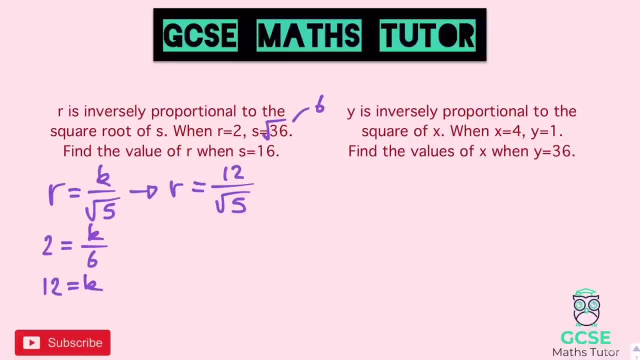 So find the value of R when S is 16.. So R equals 12 over the square root of 16.. And again the square root of 16, which can just work out to the side, just to save yourself writing down lots of stuff here. 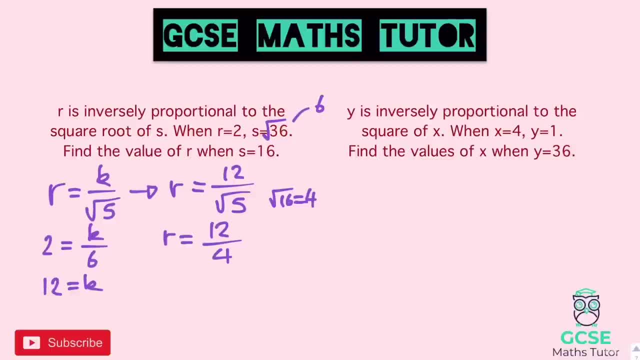 Square root of 16 equals 4.. So it's 12 over 4.. 12 divided by 4 equals 3.. So there we go. R equals 3 as our final answer On to the second one. Y is inversely proportional to. 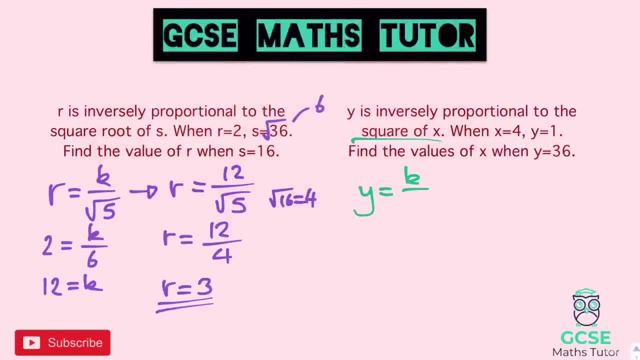 So Y equals K over the square of X, which is X squared. Plug in our values. So X is 4, Y is 1.. So 1 equals K over 4 squared. We can just work that out to the side: 4 squared equals 16.. 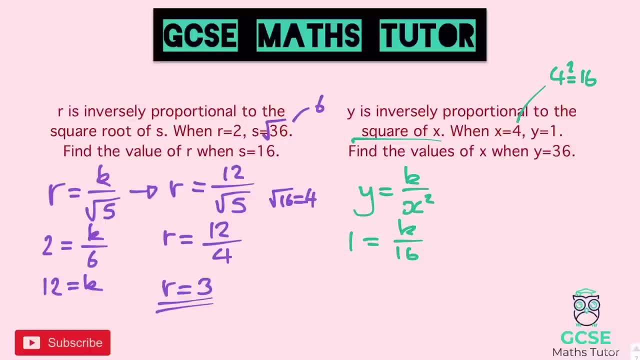 So it's K over 16.. Multiply both sides by 16 and we get 16 equals K. Exactly, Exactly the same as before. then Plug this 16 in, So we get Y equals 16 over X squared, And then find the values of X when Y equals 33.. 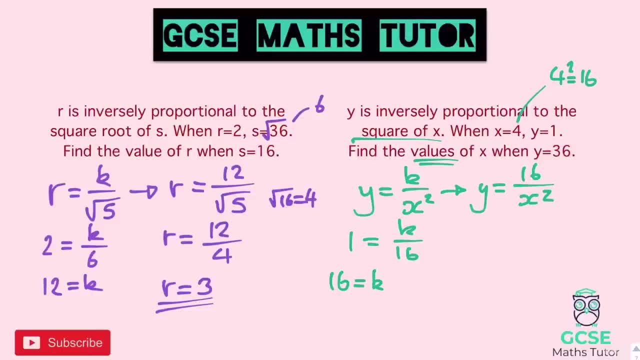 Okay, So we've got this values element coming back in again here. Hopefully you spotted that. So find the values of X when Y equals 36. So 36 equals 16 over X squared, And then again we can do our little swap here. 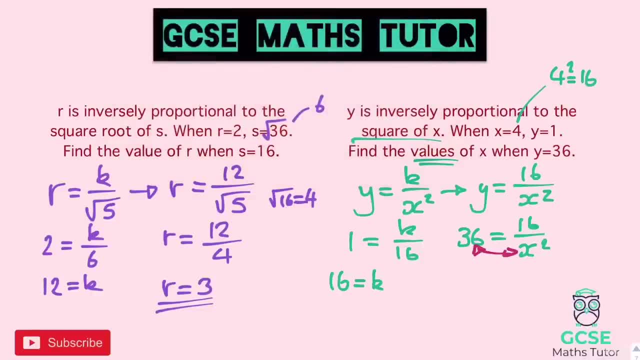 So we can swap these over. There we go And we get X squared. X squared equals 16 over 36.. Now, this is quite an interesting one, actually, because they are both square numbers And it's asking us to do the square root of this. 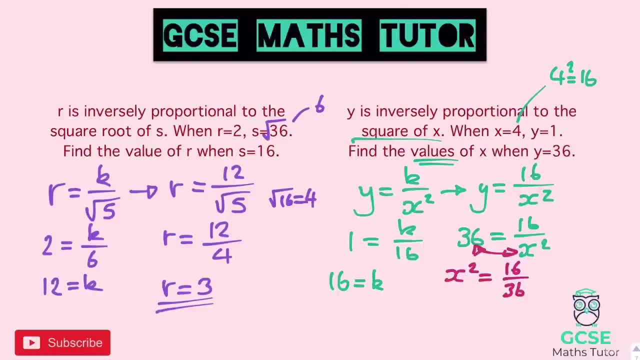 Okay, So obviously X squared equals that, So we need to square root it. So a little bit different here. Obviously, if that was a whole number, that's quite nice. Obviously, if you've got a calculator, it's very nice and easy for you to just type in your square root button. 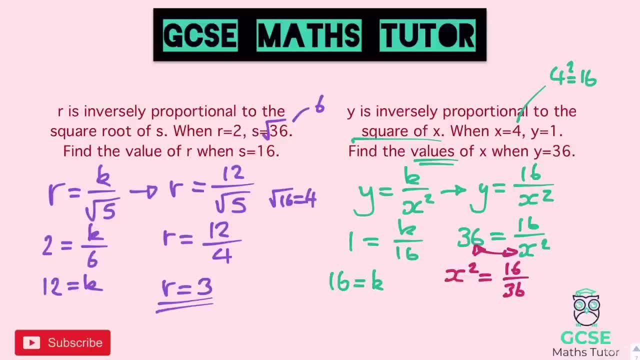 And then type in 16 over 36.. Obviously a lot easier if you have one of the dual level Casio's. Again, I'm using one of the class was's at the moment. I've linked that in the description if you are unsure on what they are. 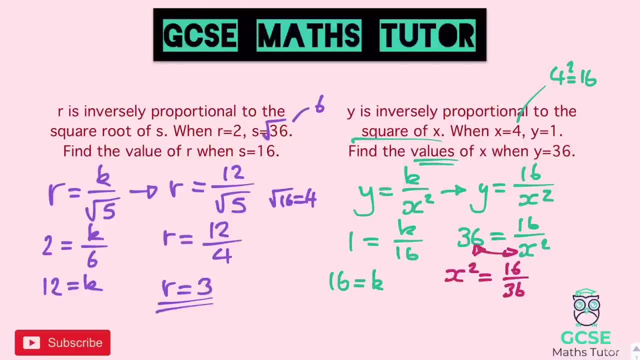 You can always have a look at them, But obviously if you type them into a calculator you get two thirds Okay, Because you need to square root the top and the bottom, And if you square root the top and the bottom you get X equals.